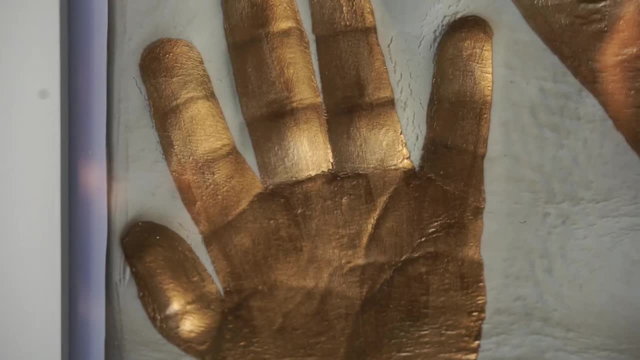 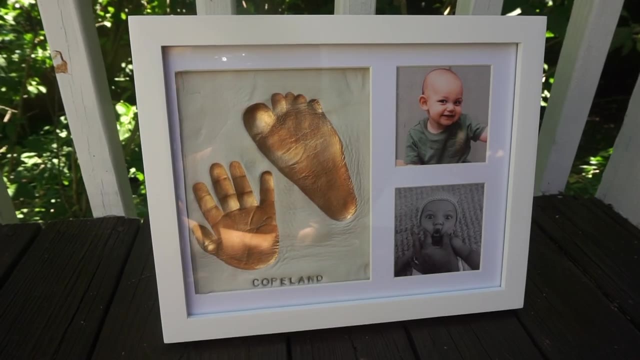 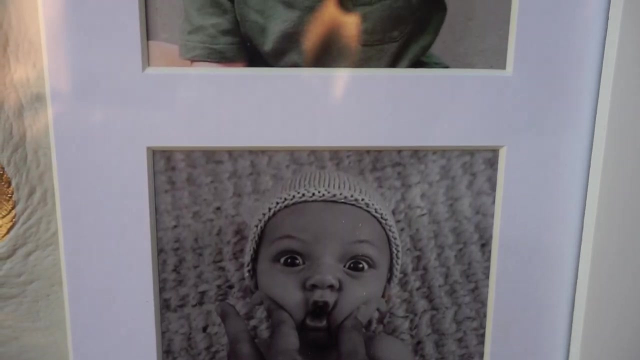 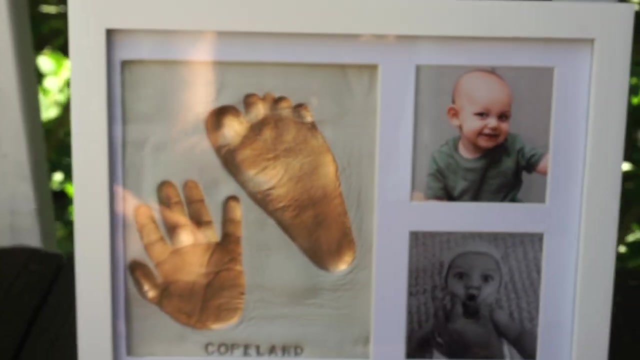 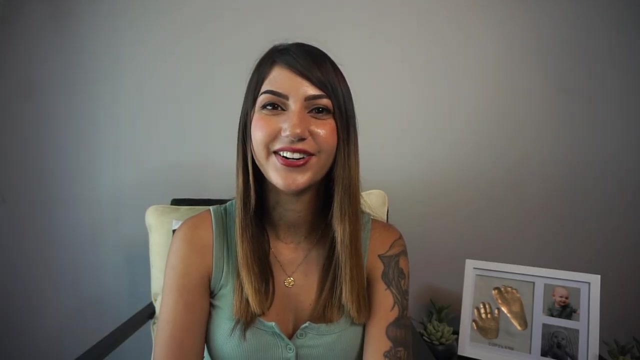 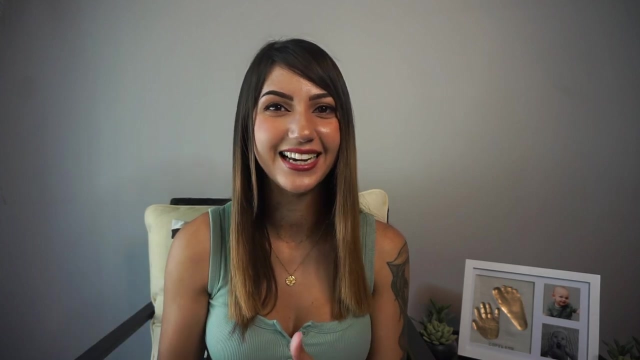 🎵. Hi guys, and welcome back to For Strong and Growing. If this is my fir- my first video, This is not my first video. If this is the first video of mine that you're seeing, thank you so much for clicking. 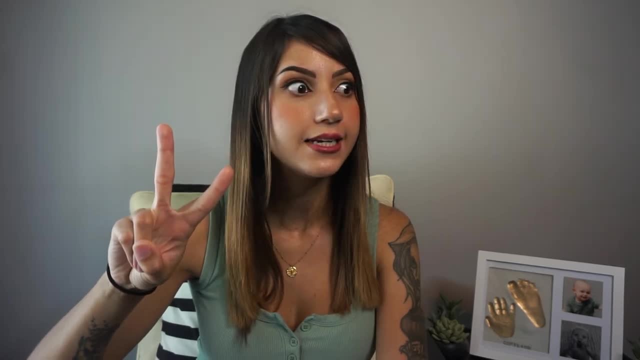 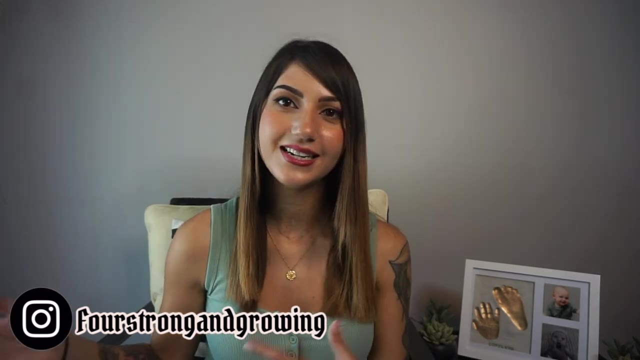 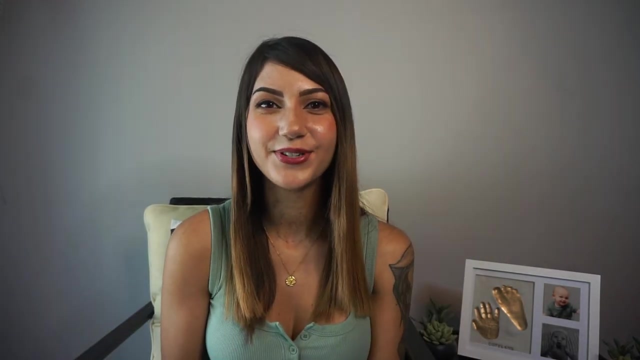 My name is Alexa and I am a mom of two crazy but amazing kiddos. This is our family channel where we document a lot of the things that go on in our lives: My pregnancies, baby updates, potty training videos, homemade baby food recipes, vlogs. a little bit of it all, But today's video is super exciting. 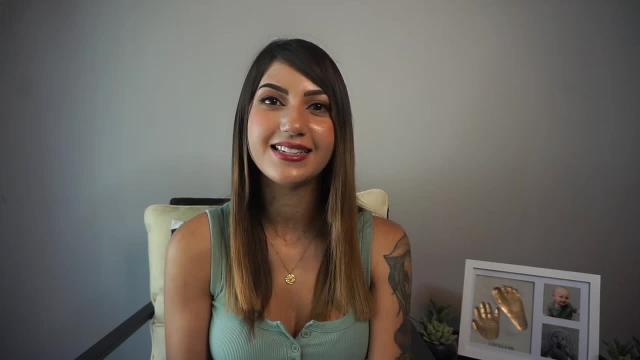 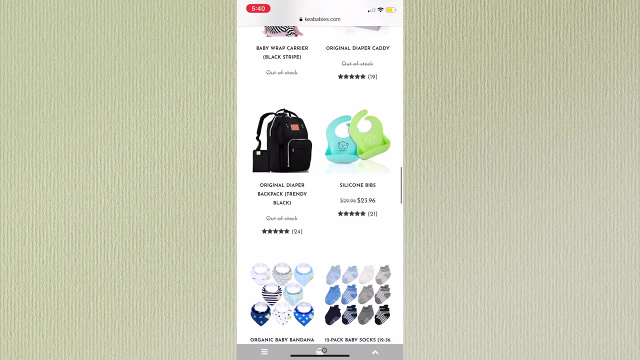 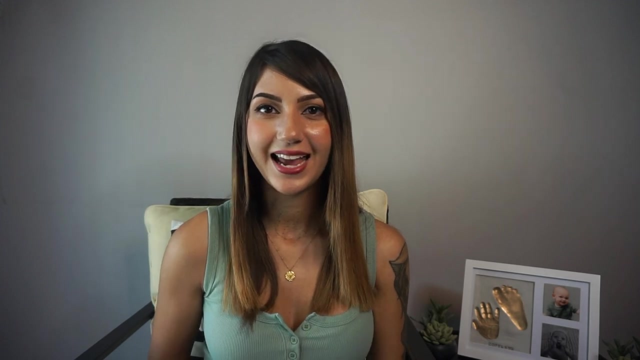 because it is in collaboration with Kia Babies. Kia Babies is a California-based company that design and sell a variety of baby products, Anything from really cute diaper bags to baby wraps, bibs, baby accessories and some really cute keepsake kits. They reached out to me and 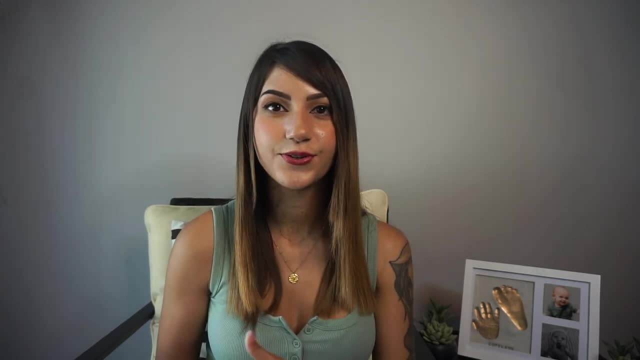 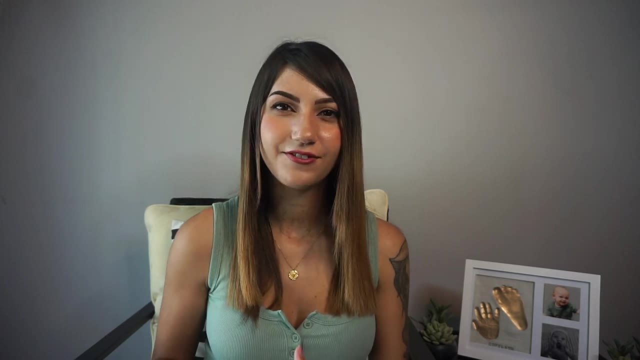 allowed me to pick any item off of their website to review, and I chose their Baby Clay Handprint Footprint Keepsake Kit. This is a kit that's designed to perfectly capture the details of your baby's tiny hands and feet and display them in a clay mold that you can personalize. 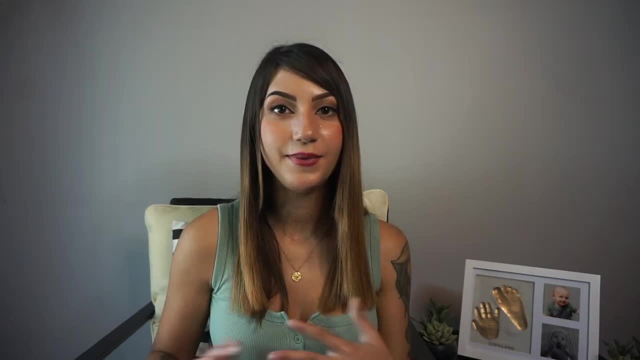 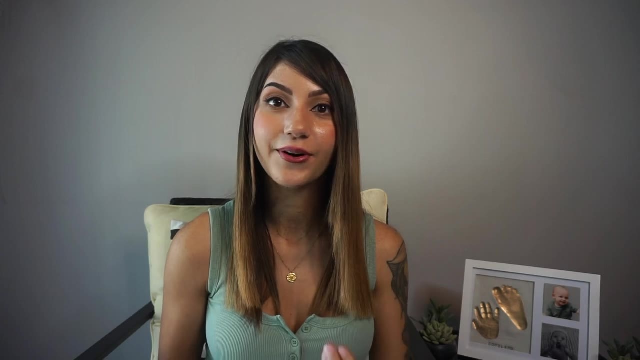 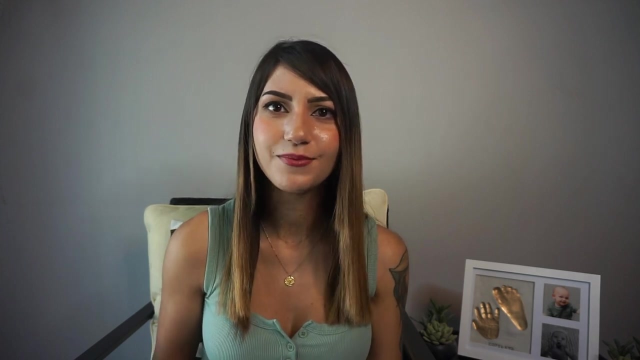 decorate yourself, frame and then display. This kit immediately stood out to me while I was looking through their products, because me and my fiancé Matt were just literally talking about how our son, Copeland, is about to turn one year old, on August 14th, and that we need something to document this. 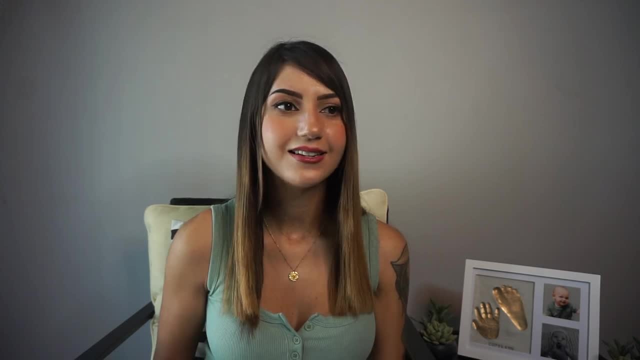 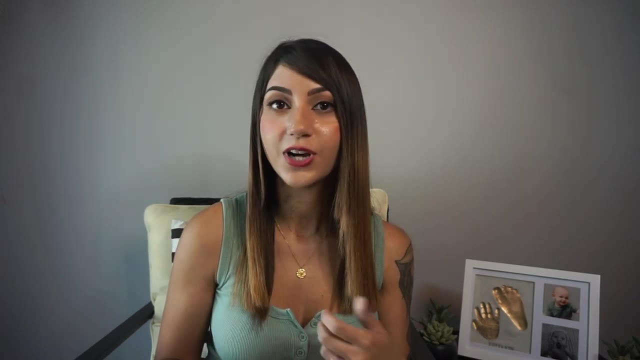 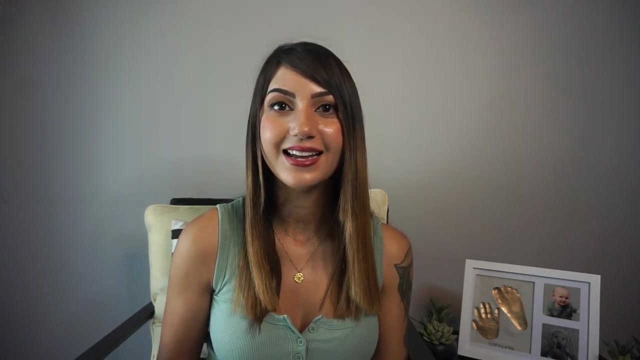 time of our lives Like this year has gone by so fast and we have digital pictures on our phones and computers, but we wanted some sort of physical keepsake to document this time in our lives, So this was an easy pick. We definitely discovered this product at the perfect time, and I'm really 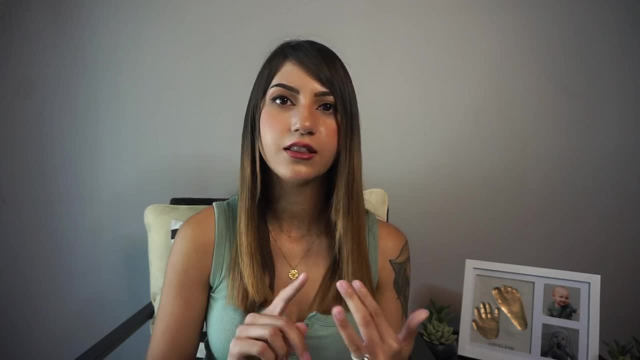 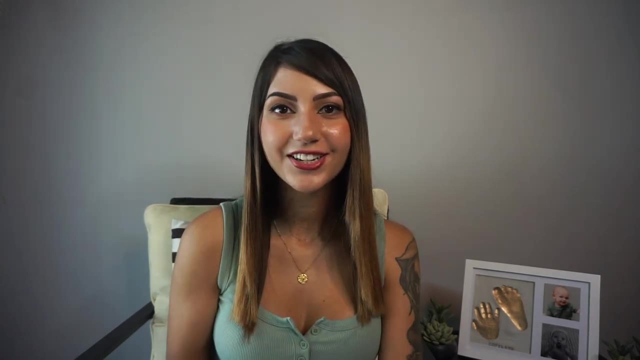 excited to give you guys an honest review of the packaging, the quality, the ease of actually using this product and basically whether or not I think it's worth it for you to purchase. So I actually filmed myself from start to finish using this product. I did an unboxing. I show you exactly. 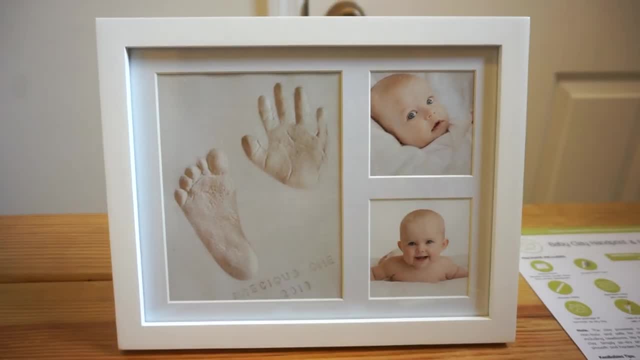 how everything came in the first place. So I'm going to show you how everything came in the first place in the package and filmed myself using it. So if you're interested in seeing how I made a really adorable keepsake for my son, just keep on watching. 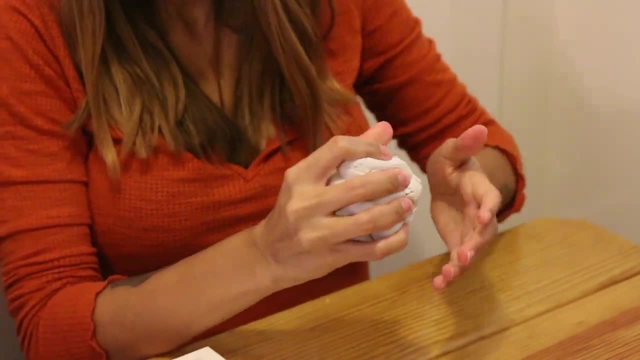 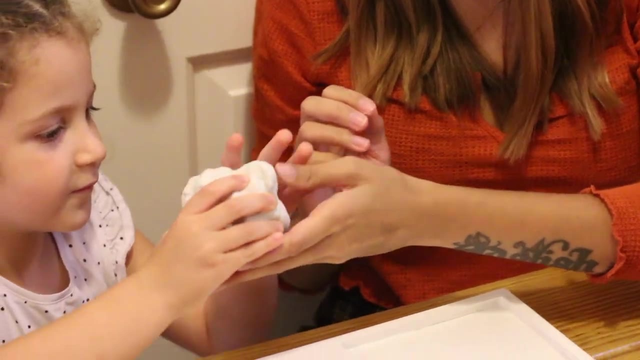 So I'll be showing you guys how the STALID looks like after I put it on and take a look at it. So you are going to want to have a few pictures on you that you can put together for the next. 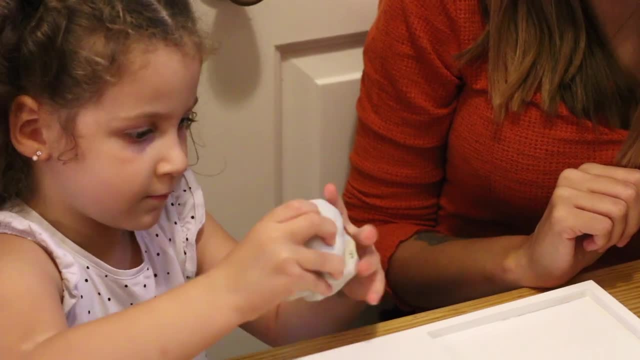 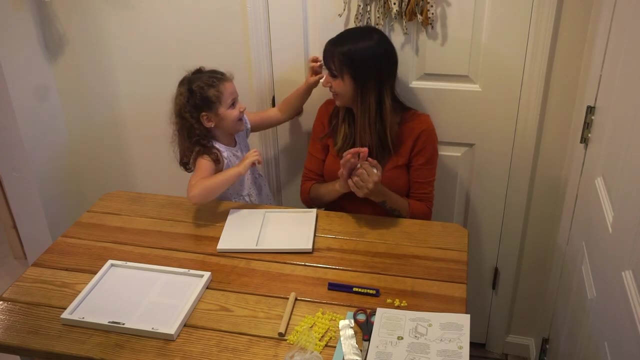 time you're looking at this And we want to make it look like a real, really cute, very cute, very cute, very cute keepsake. So let's go ahead and double check and see what we've got. So here's a picture of what we've got. 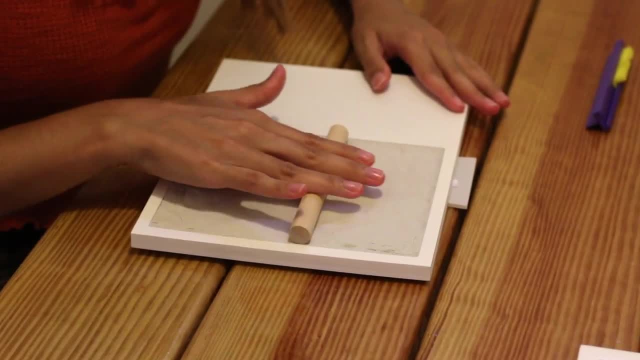 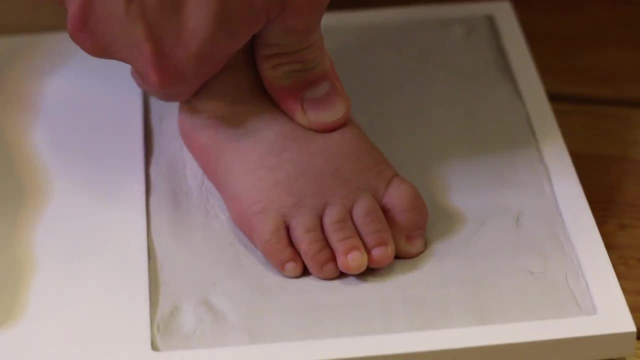 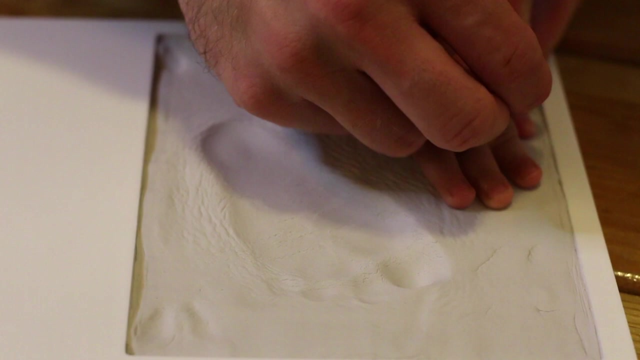 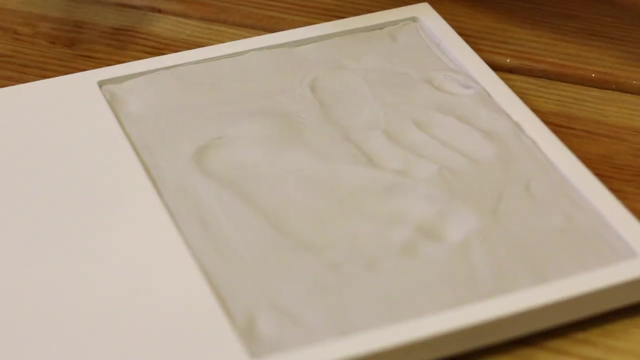 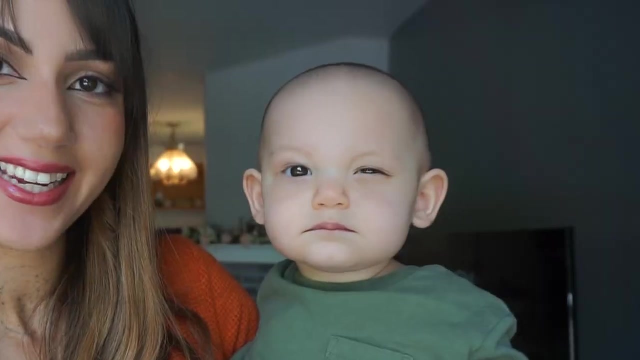 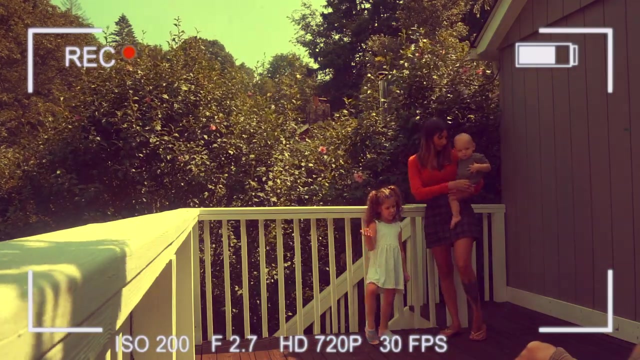 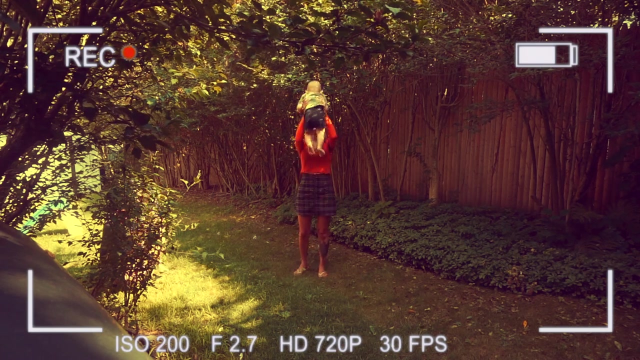 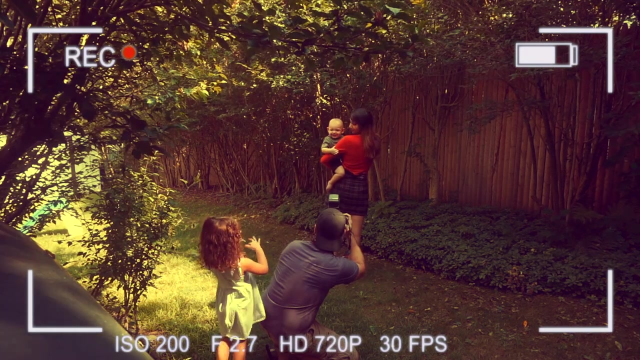 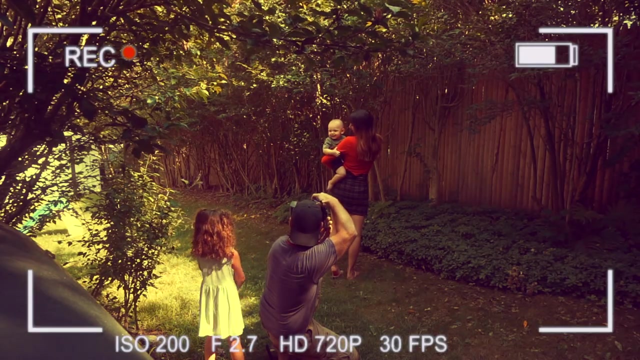 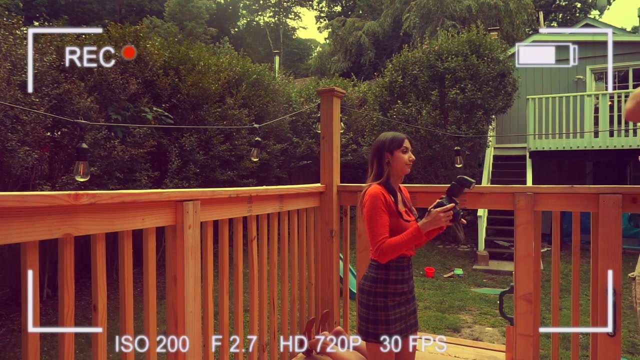 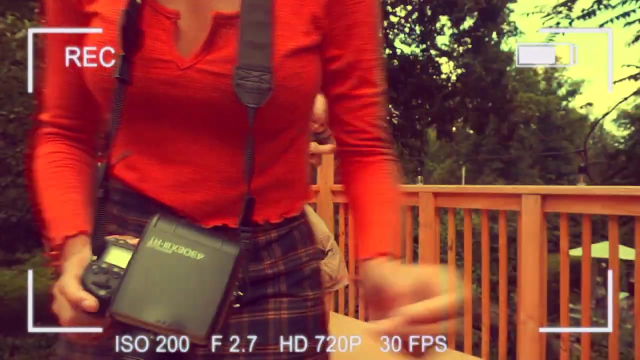 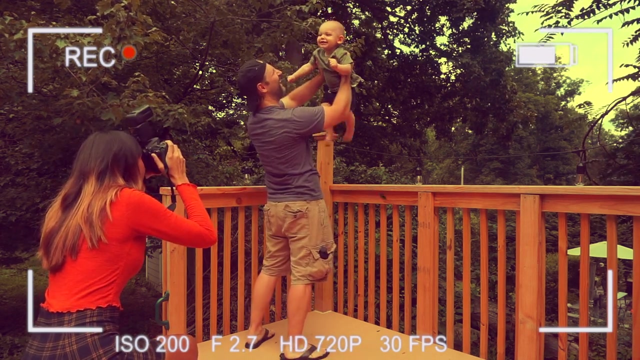 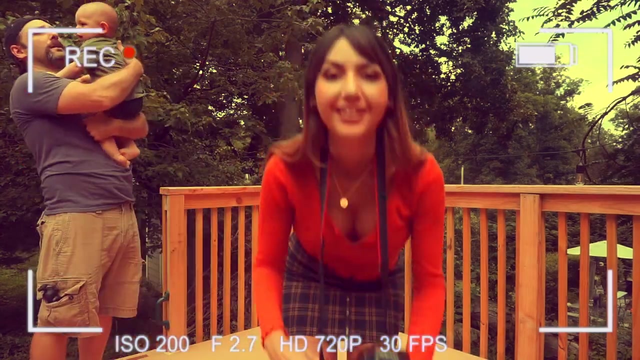 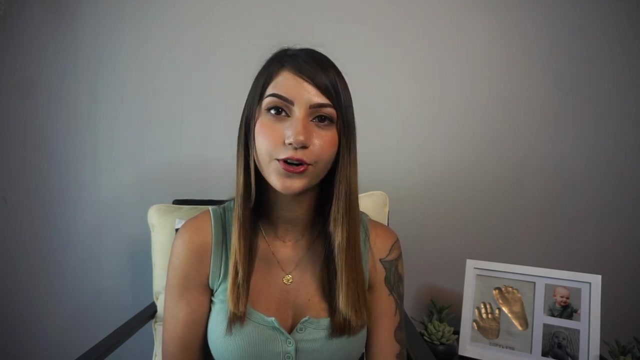 Ready for your photo shoot. You're looking so handsome. look at you. You're looking so handsome, look at you, Hi guys, okay, so it is five days later. The instructions say to let the clay dry for four days before painting it or framing it. 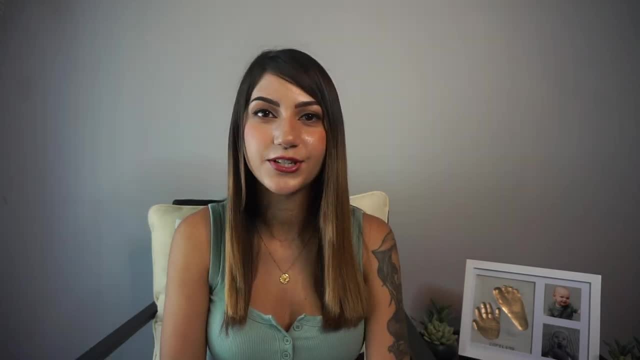 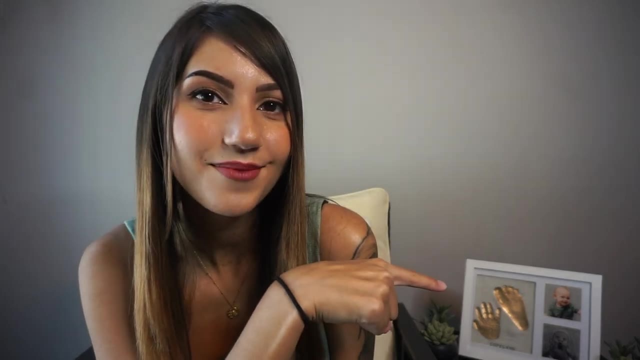 so that is exactly what I've done, And now that I am completely done with this project, I think it's time to give my final thoughts. And, in case you haven't seen, it's on the table right there. It looks so good guys. 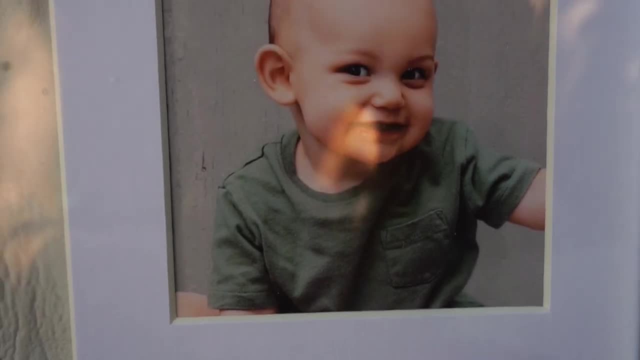 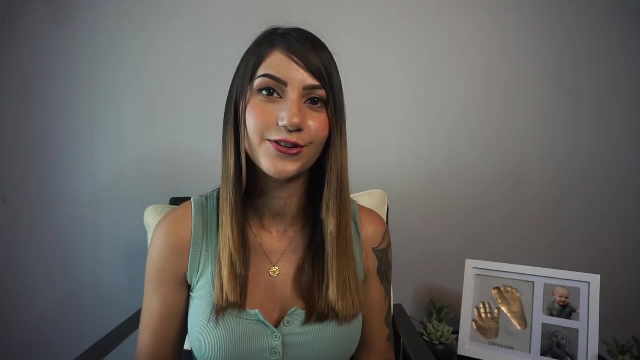 I am really pleasantly surprised at how nice this turned out. It is so cute, It's so personalized And I just can't wait to actually be done with this video so that I can go hang it up. So, to start off, the shipping was really fast. 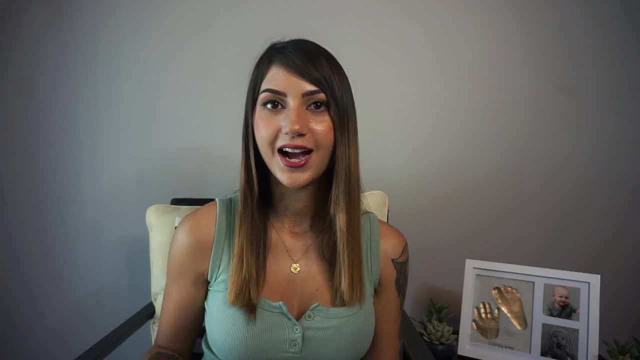 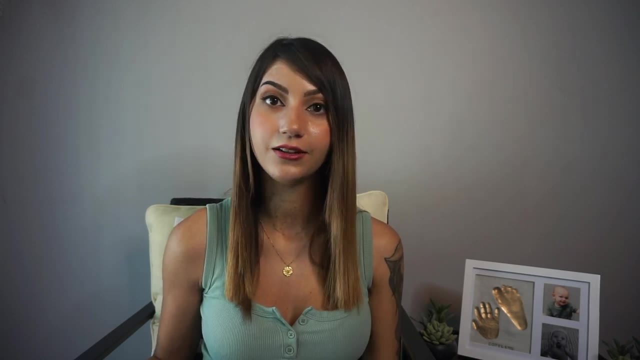 I only had to wait a few days to get this in the mail. When it arrived, everything was in good condition. Nothing was broken. Everything that was supposed to be included in the kit was included. The frame and the glass were both protected by a layer of bubble wrap and then a second. 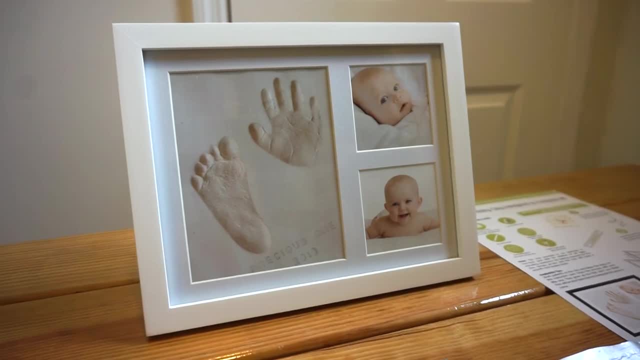 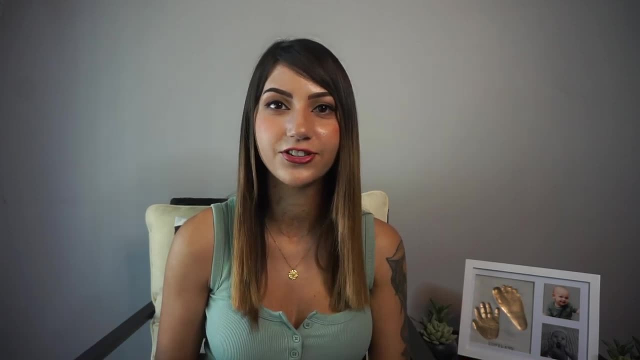 layer. that wasn't bubble wrap, but it was a different type of material to protect it. The frame fit very nicely into the box. There wasn't a lot of wiggle room, which means that it wasn't bouncing around during transit. So everything checks out for packaging. 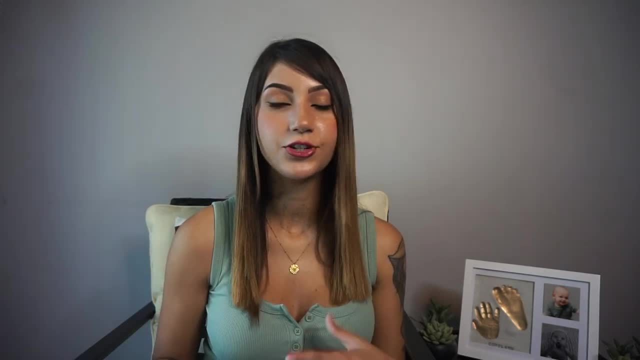 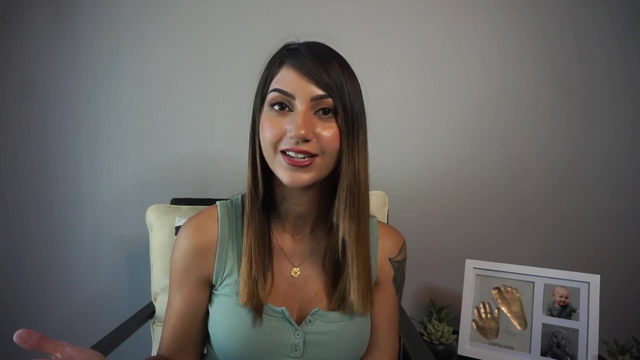 As far as the ease of actually doing this project, the directions were really easy to follow. I really appreciate There is a link to video instructions as well as the written instructions, So that was really helpful to actually see a mini tutorial of how to do this before actually. 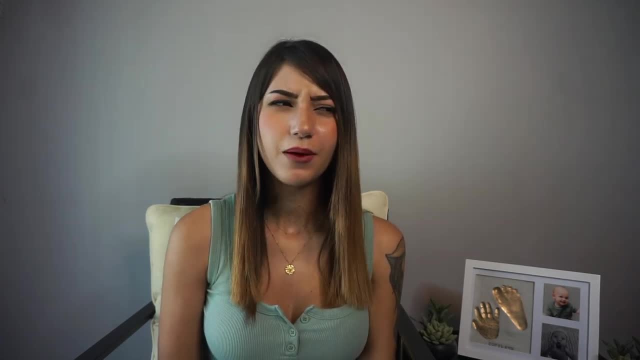 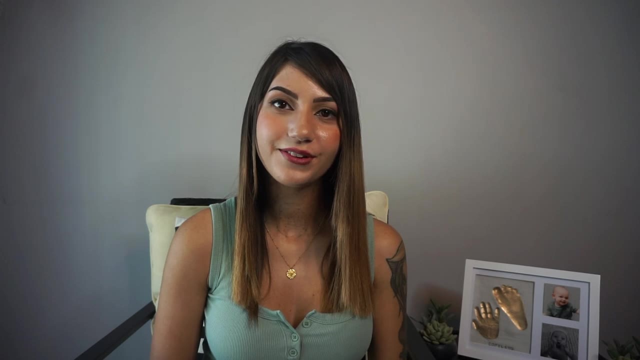 attempting it. I would say it is a two person project. You probably could do it alone if you're determined enough, but I think it would definitely be easier with two people. The most difficult part of this project was getting the clay to smooth out. 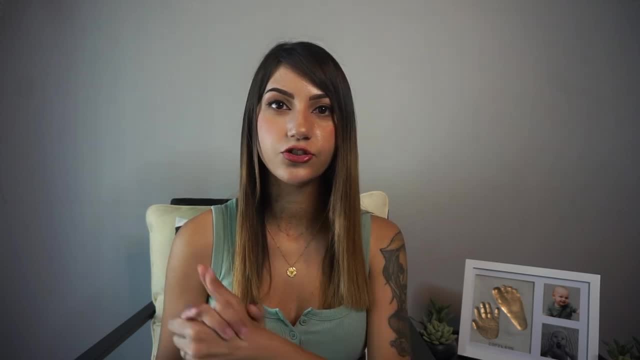 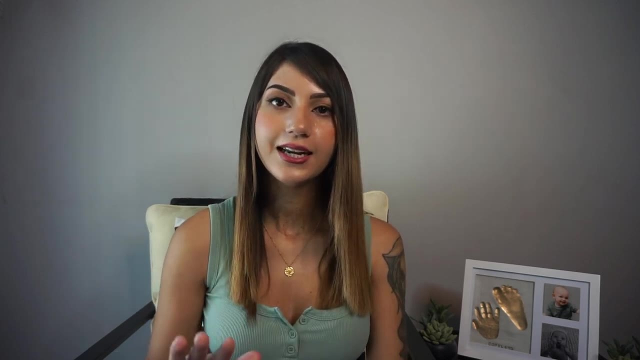 This actually took me two attempts. The first time, I took the clay straight out of the package and I kneaded it for about four or five minutes in my hands and then rolled it out very slowly. And what I didn't realize is that by going so slow it was actually starting to dry and 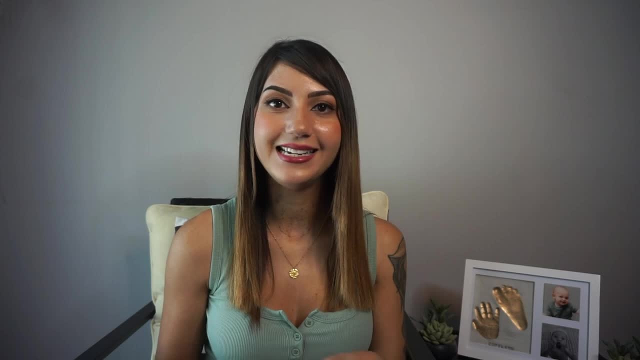 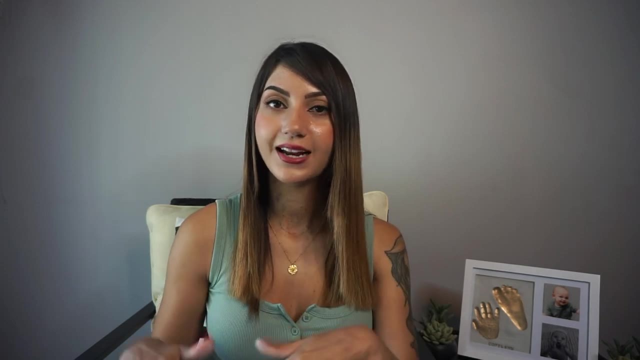 crack. So what I ended up doing second time around was kneading in a little bit of all the clay. I added a little bit of olive oil into the clay and this kept it nice and moist, And then I worked pretty quickly to spread it out and roll it down nicely into the tray. 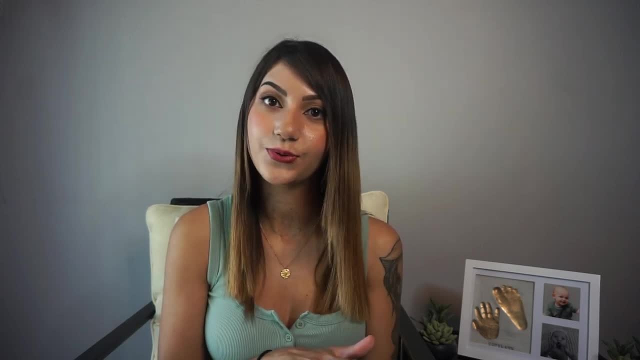 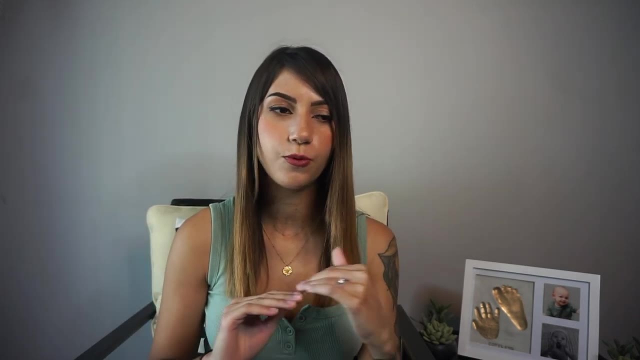 and then quickly stamping his feet and hands into it before it had time to dry and crack. So, pro tip, add a little bit of olive oil into your clay and it will make a world of a difference. After we did that, we had a beautiful blank canvas to work on, and it gave us really nice. 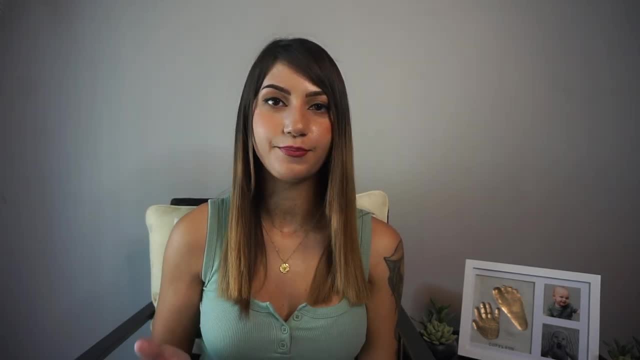 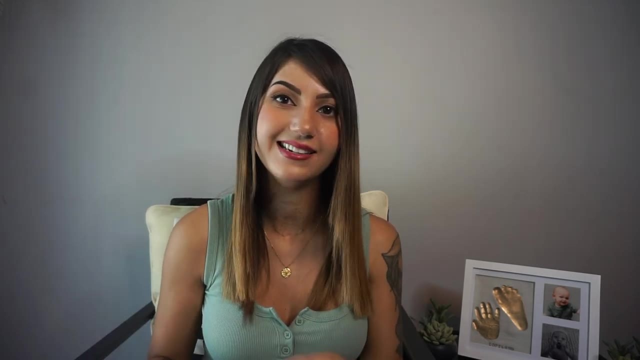 end results. And another tip is to make sure that whatever you're stamping is as close together as you can, As close to center as you can get it, because if you go too far off to the sides of the clay, it's going to get cut off by the interior frame. 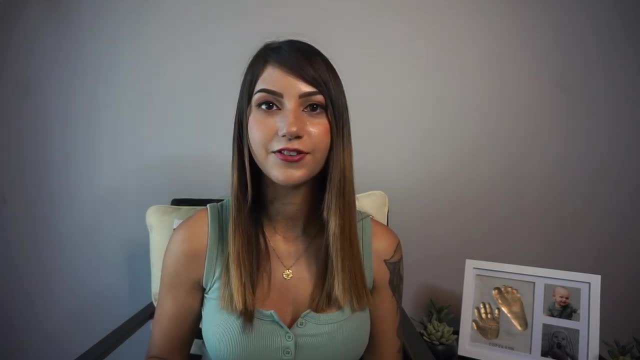 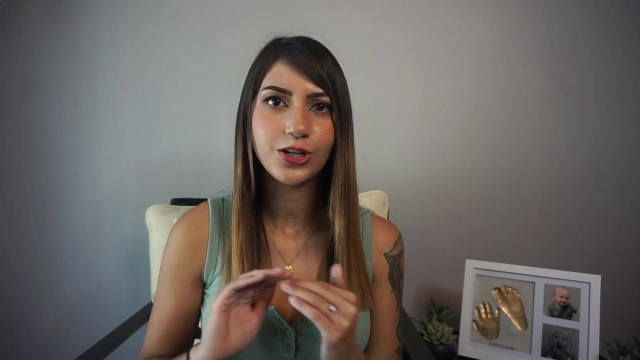 The gold paint is what I think kind of sets this product apart from other brands who have similar products that I've seen. I haven't seen anyone else who includes gold paint with the kit and I actually think it makes a huge difference. When you paint the clay it actually shows more of the details in the hand or foot. 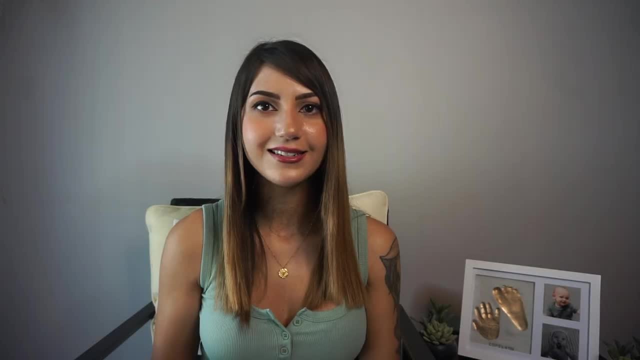 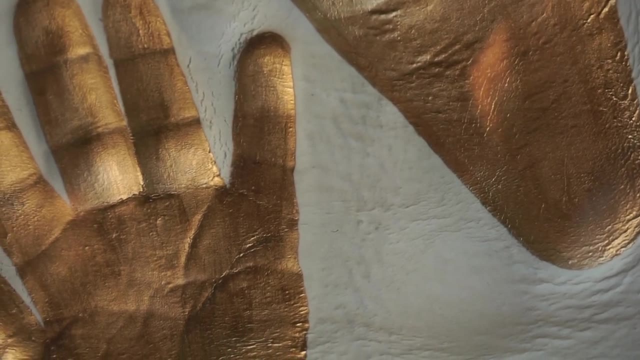 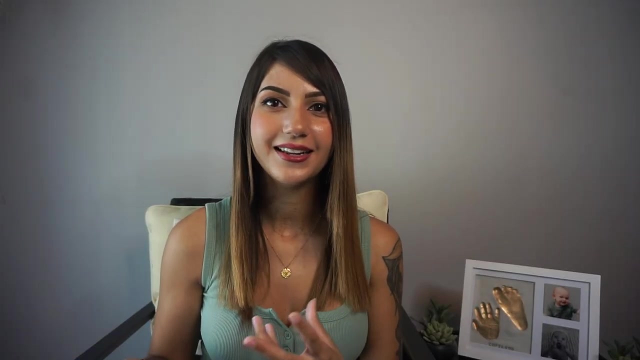 The paint accentuates those little lines and creases and it kind of creates a sort of optical effect where it appears that the hand or foot is coming out 3D instead of actually being sunken in. I'm not sure why or how that happens, but that's the effect that comes off and it's so cool. 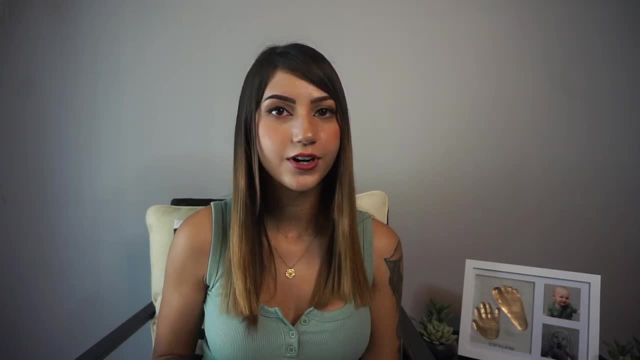 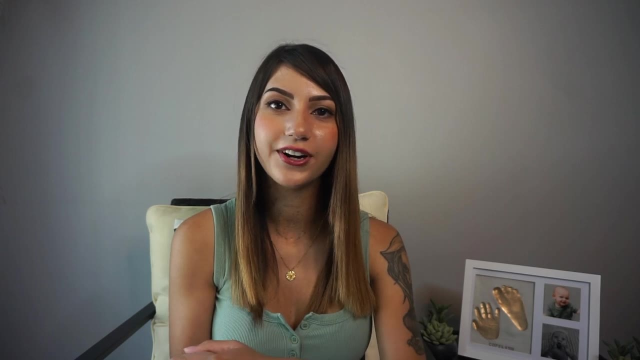 And on top of that, gold and white are two of my favorite decor colors, so this perfectly matches the rest of the decor in my house. I definitely think that this kit is worth it, especially for the quality of product that you're receiving at a really reasonable price point. 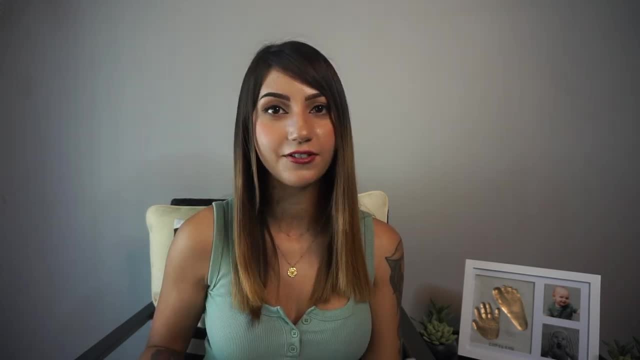 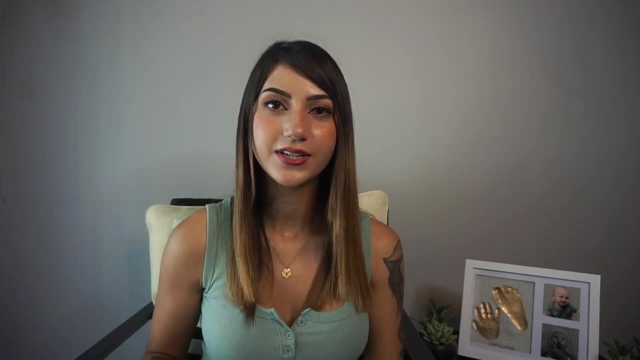 Nowadays it's so easy to only have digital memories of our little ones, but I don't want to lose sight of the importance of actual physical keepsakes. I really like that we're not only going to have the memory of Copeland in this season. 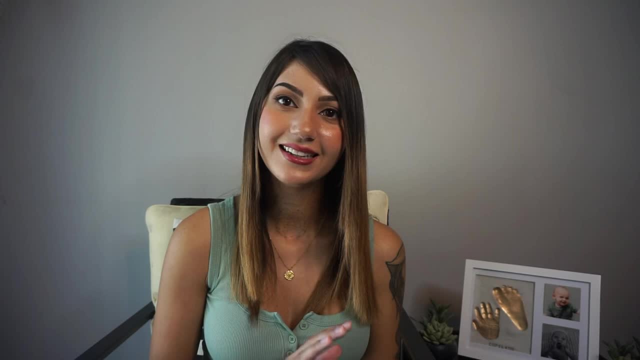 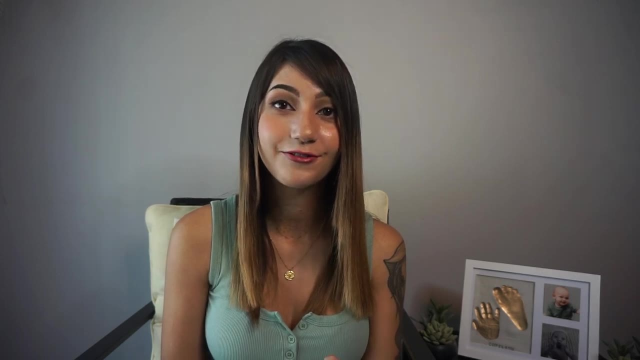 of his life. but we also have the memories of actually making the keepsake, And one thing I wasn't able to catch on camera is that he actually puked onto the corner of the clay the first time we tried to stamp his foot. 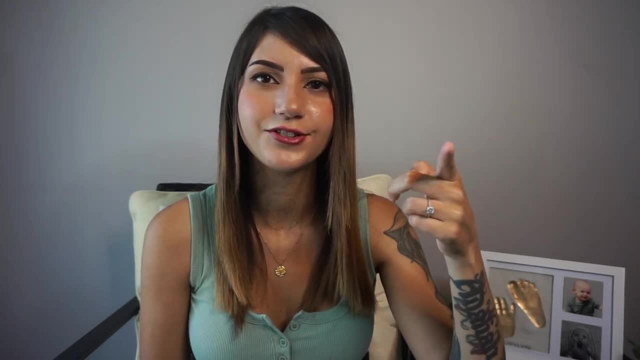 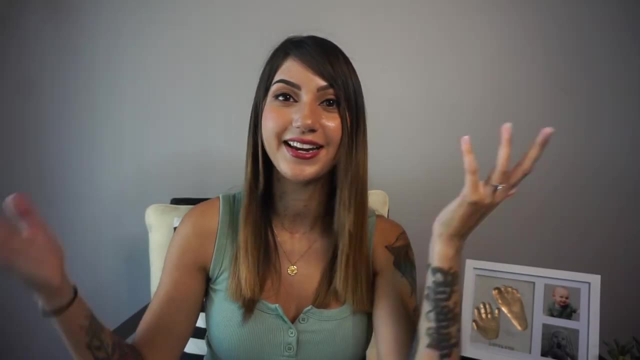 Of course he did. Why wouldn't he? Another pro tip: Don't push your baby directly after you feed your baby dinner. Really, just don't push on their belly when you're holding them over the clay. Which I probably should have known, but here I am. 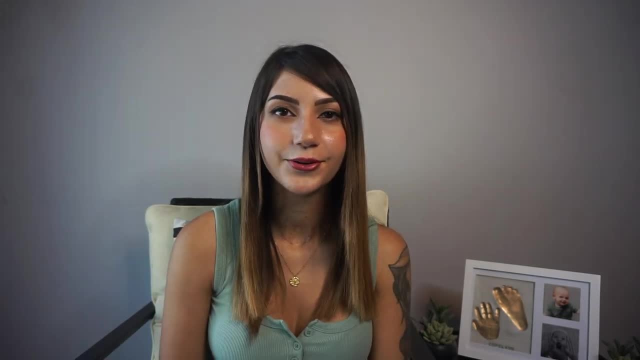 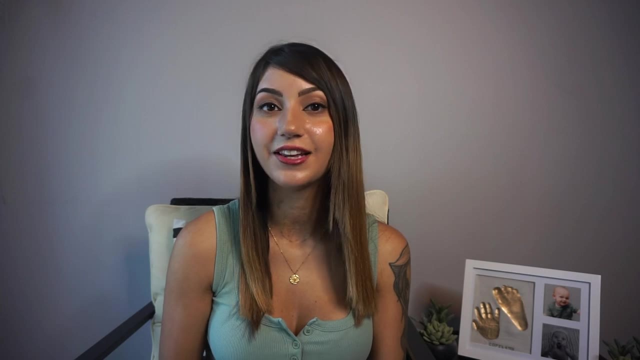 So it was a little chaotic, but, to be honest, I wouldn't have it any other way. So I definitely recommend this to anyone with a baby under the age of two, and if you don't, I still feel like it would be a really thoughtful baby shower gift or a gift to new parents. 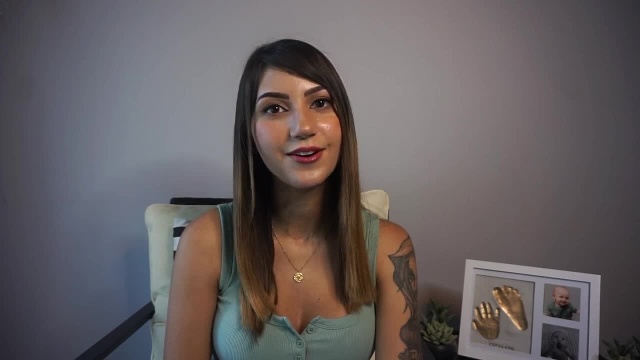 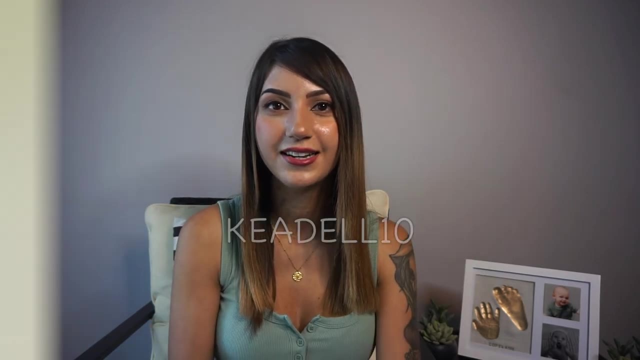 I asked Kia Babies if they would be willing to offer my followers a discount, and they were kind enough to give you guys 10% off of your order using the code on the screen, and I will also link it in the description.